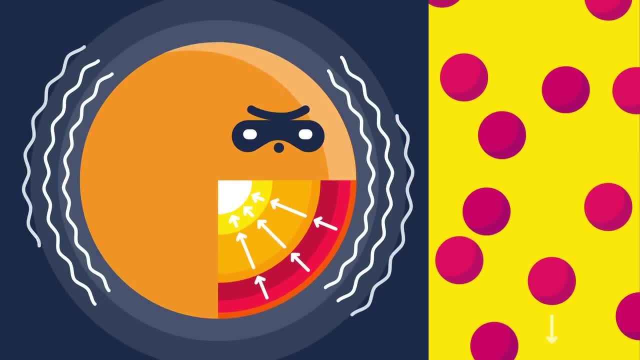 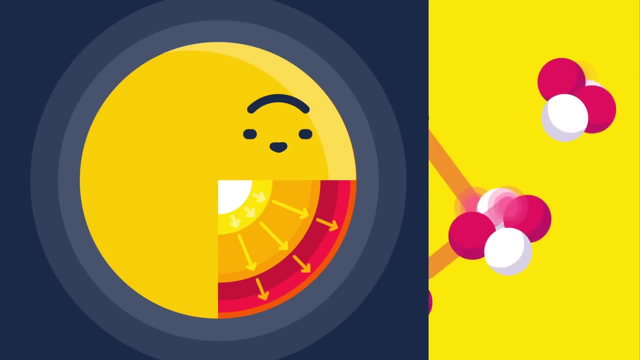 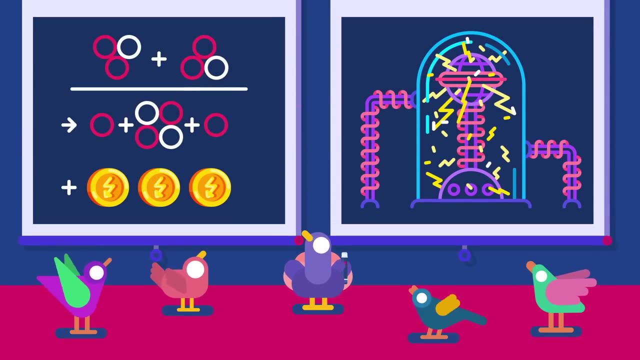 They are so massive that the pressure in their cores generates the heat to squeeze the nuclei together until they merge and fuse, creating heavier nuclei and releasing energy in the process. It is this energy release that scientists hope to harness in a new generation of power plant: the fusion reactor. 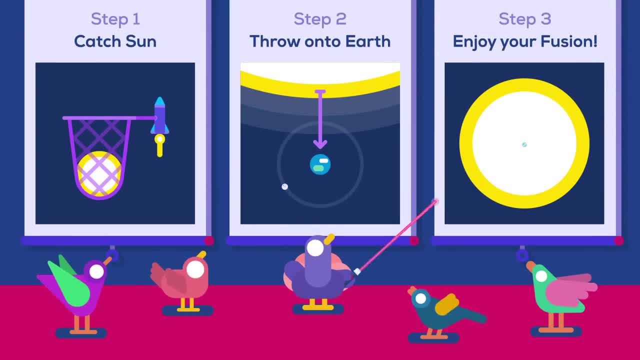 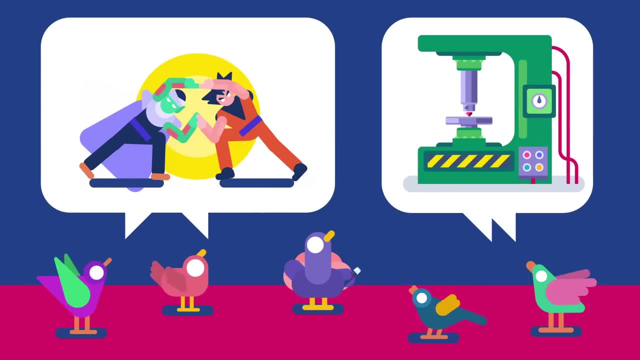 On Earth, it's not feasible to use this brute force method to create fusion, so if we wanted to build a reactor that generates energy from fusion, we have to get clever. To date, scientists have invented two ways of making plasmas hot enough to fuse. 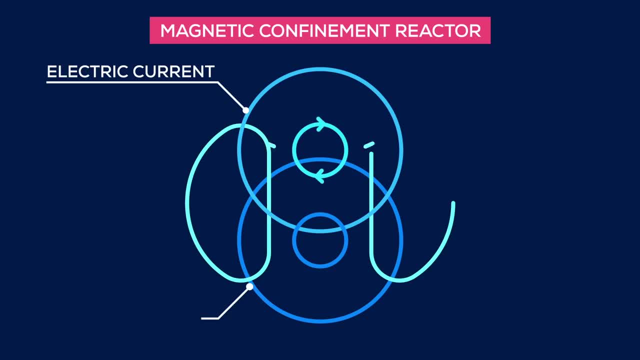 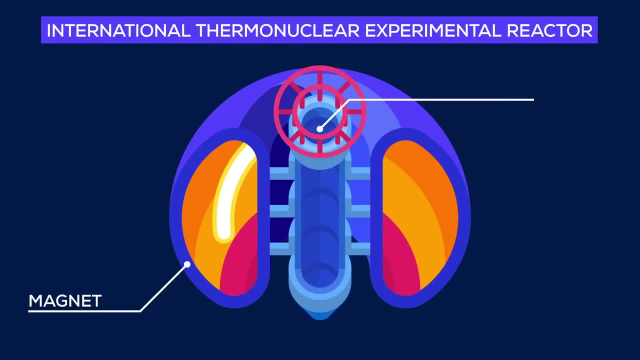 The first type of reactor uses a magnetic field to squeeze a plasma in a doughnut-shaped chamber where the reactions take place. These magnetic confinement reactors, such as the ITER reactor in France, use superconducting electromagnets cooled with liquid helium to within a few degrees of absolute zero. 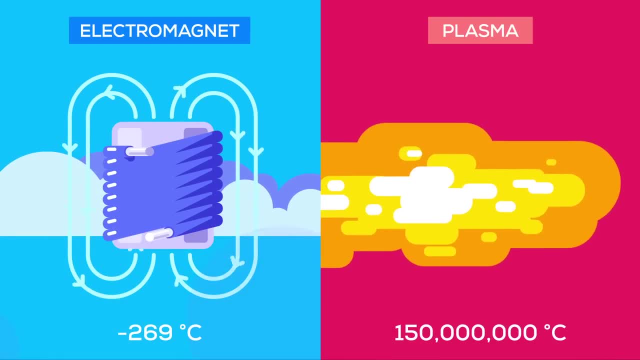 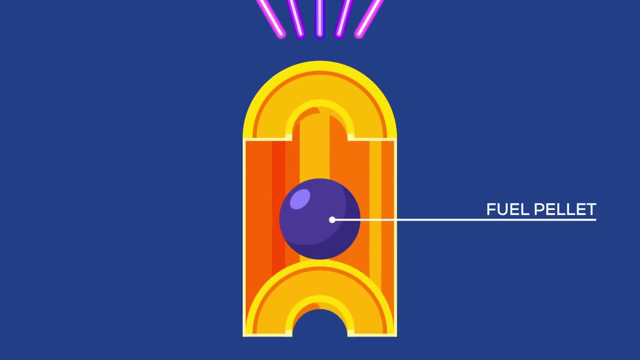 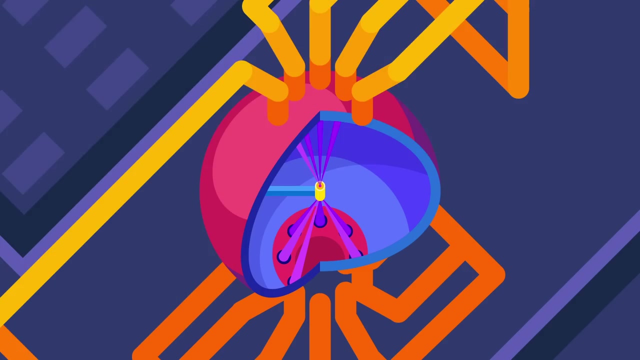 meaning they host some of the biggest temperature gradients in the known universe. The second type, called inertial confinement, uses pulses from superpowered lasers to heat the surface surface. These pulses produce massive appellas of fuel, imploding it briefly, making the fuel hot and dense enough to fuse. 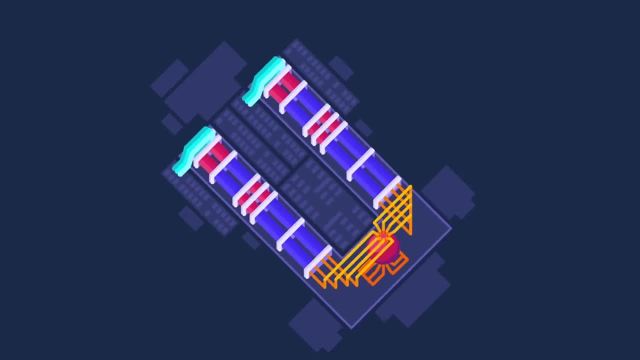 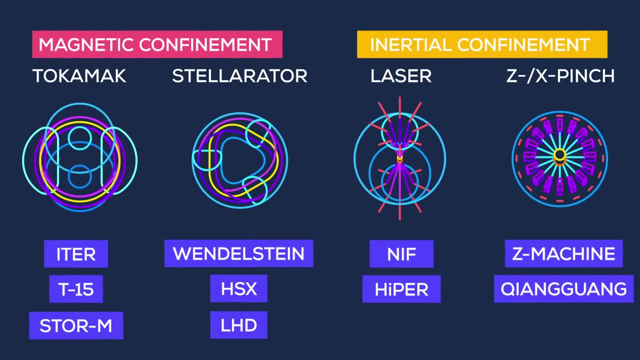 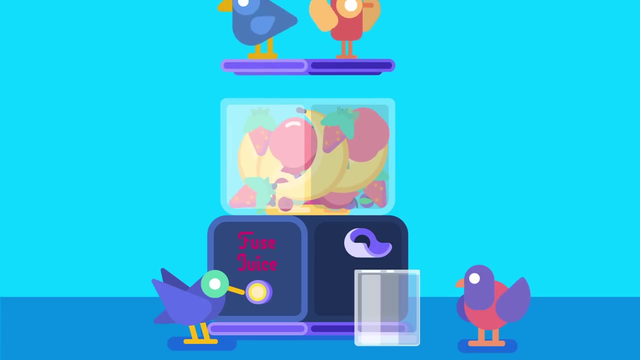 In fact, one of the most powerful lasers in the world is used for fusion experiments at the National Ignition Facility in the US. These experiments, and others like them around the world, are today just experiments. Scientists are still developing the technology And although they can achieve fusion, 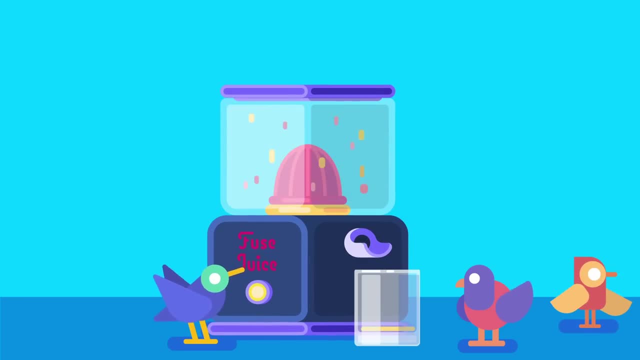 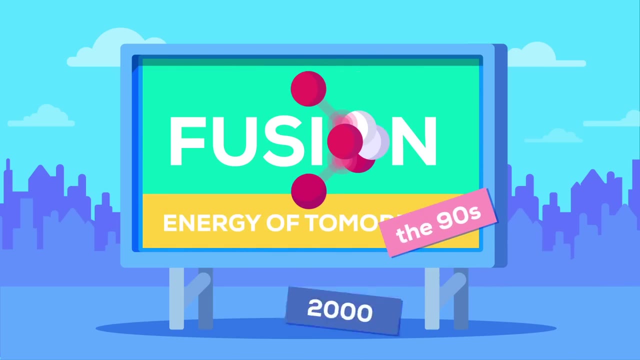 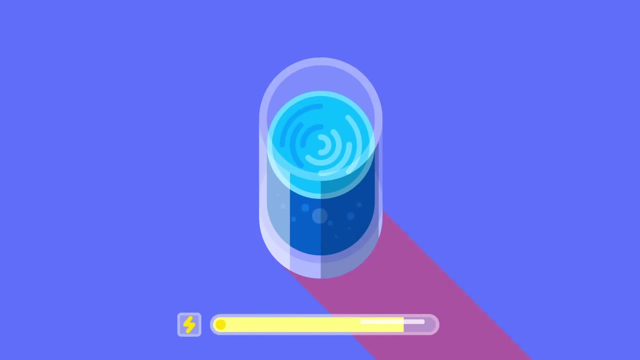 right now it costs more energy to do the experiments. The technology has a long way to go before it's commercially viable, And maybe it never will be. It might just be impossible to make a viable fusion reactor on Earth, But if it gets there it would be so efficient. 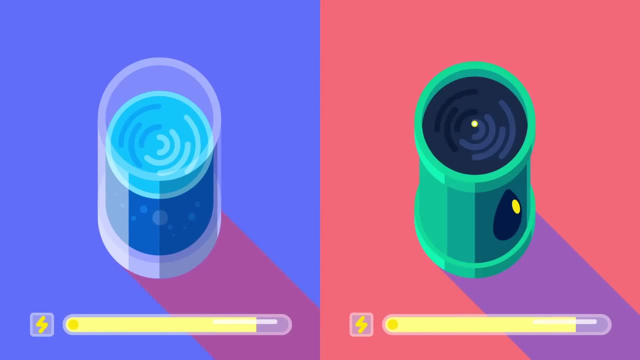 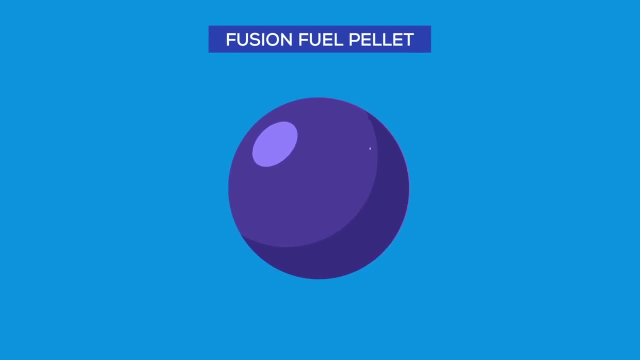 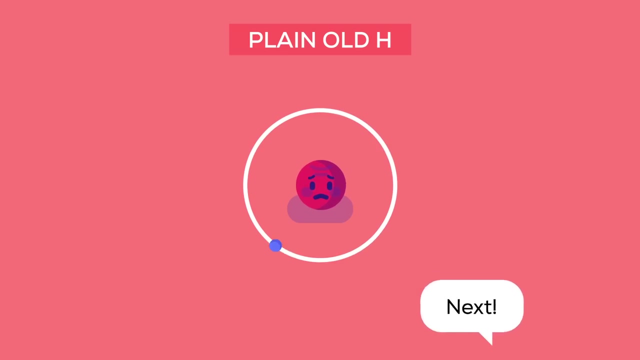 that a single glass of seawater could be used to produce as much energy as burning a barrel of oil, with no waste to speak of. This is because fusion reactors would use hydrogen or helium as fuel, and seawater is loaded with hydrogen, As any hydrogen will do. 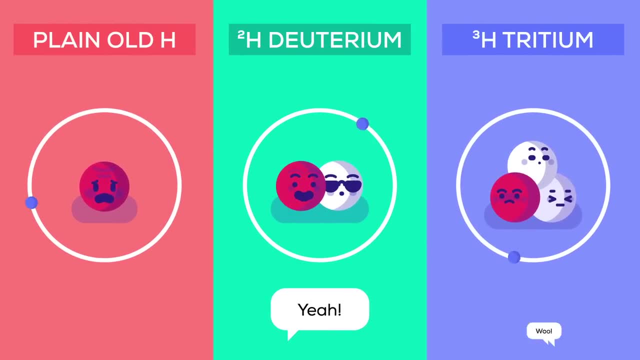 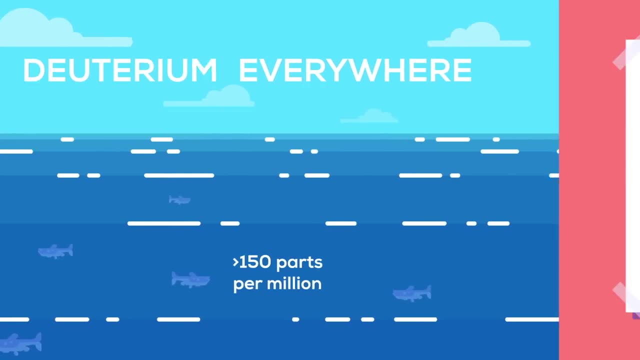 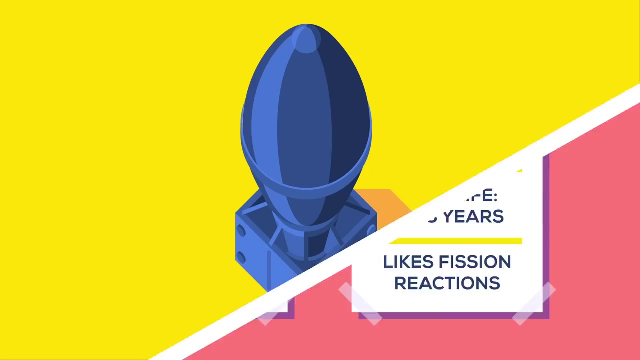 specific isotopes with extra neutrons called deuterium and tritium are needed to make the right reactions. Deuterium is stable and can be found in abundance in seawater, though tritium is a bit trickier: It's radioactive and there may only be 20 kilograms of it in the world. 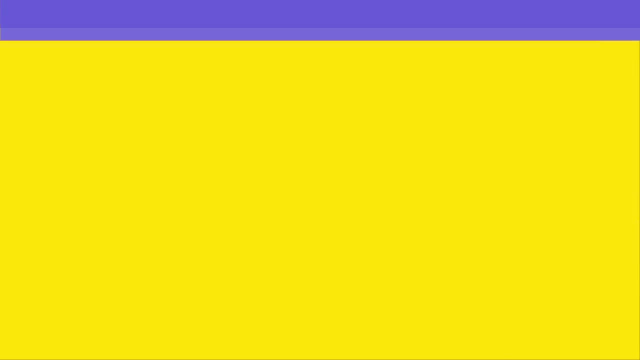 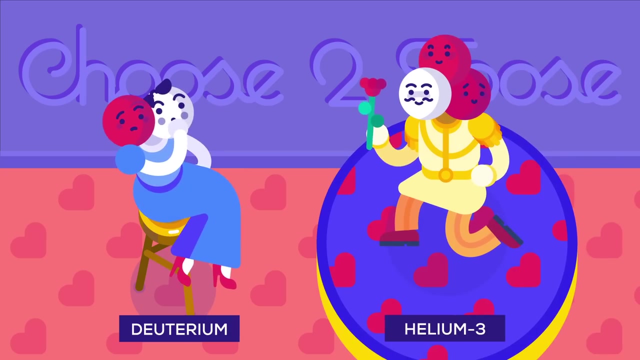 mostly in nuclear warheads, which makes it incredibly expensive. So we may need another fusion buddy for deuterium instead of tritium Helium-3,, an isotope of helium might be a great substitute. Unfortunately, it's also incredibly rare on Earth. 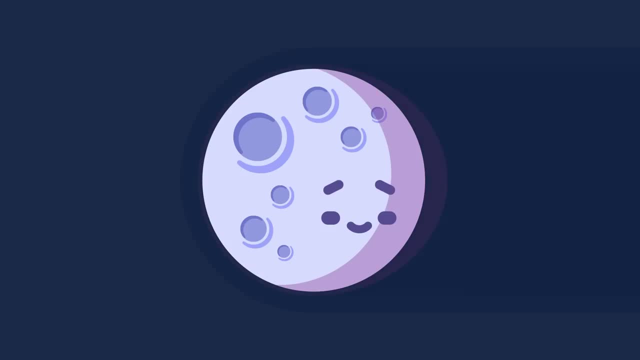 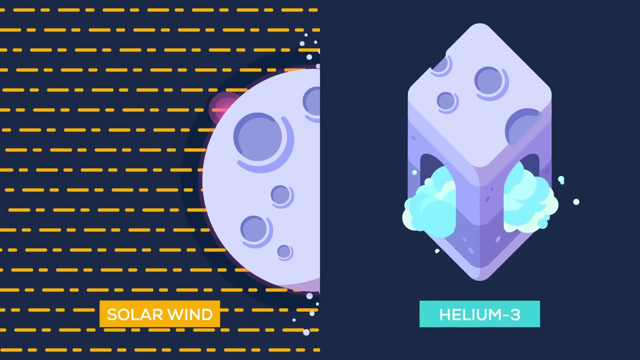 But here the Moon might have the answer. Over billions of years, the solar wind may have built up huge deposits of helium-3 on the Moon. Instead of making helium-3, we can mine it If we could sift the lunar dust for helium. 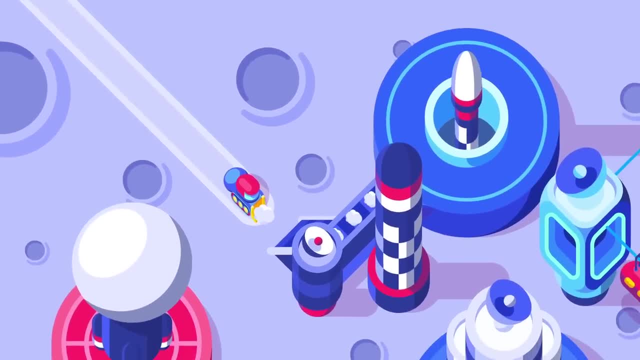 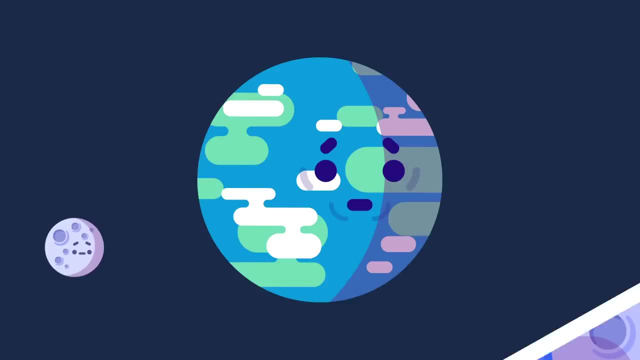 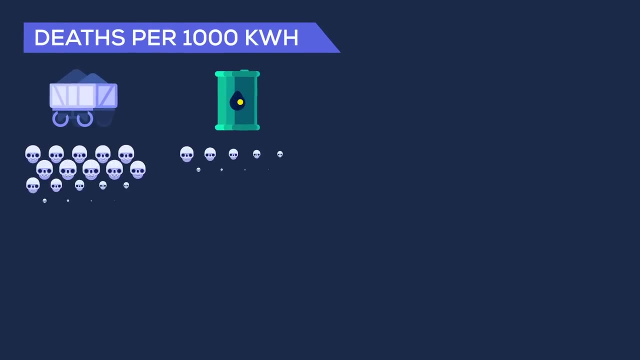 we'd have enough fuel to power the entire world for thousands of years. One more argument for establishing a Moon base, if you weren't convinced already. Okay, maybe you think building a mini-Sun still sounds kind of dangerous, But they'd actually be much safer than most other types of power plant. 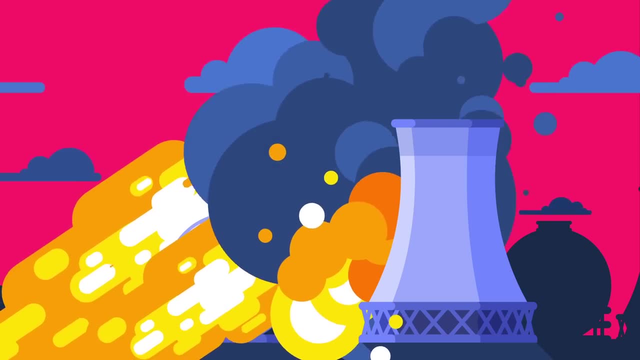 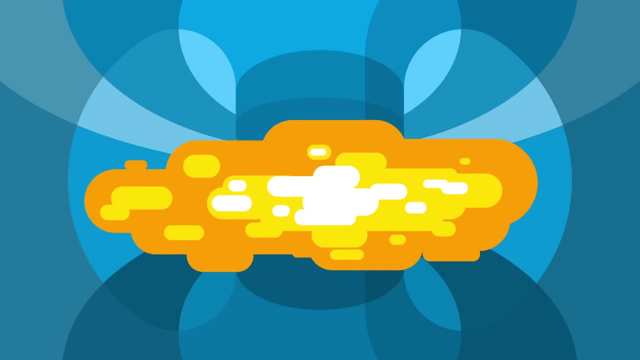 A fusion reactor is not like a nuclear plant which can melt down catastrophically. If the confinement failed, then the plasma would expand and cool and the reaction would stop. Put simply, it's not a bomb. The release of radioactive fuel. 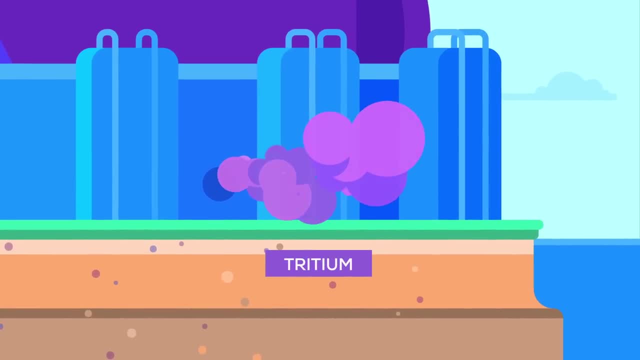 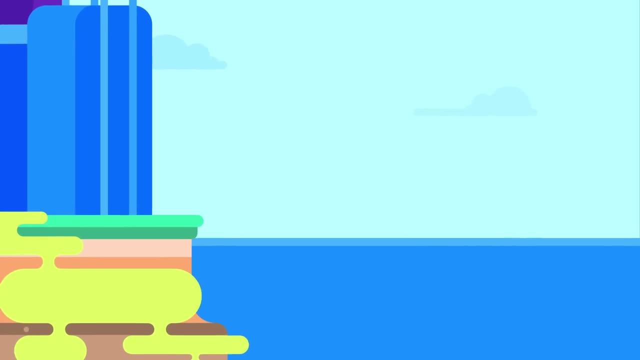 like tritium, could pose a threat to the environment. Tritium could bond with oxygen-making radioactive water, which could be dangerous as it seeps into the environment. Fortunately, there's no more than a few grams of tritium in use at a given time. 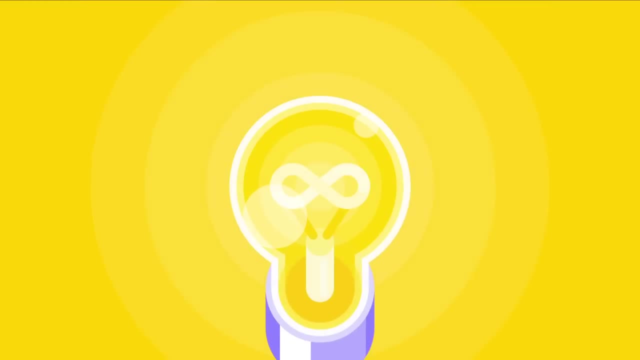 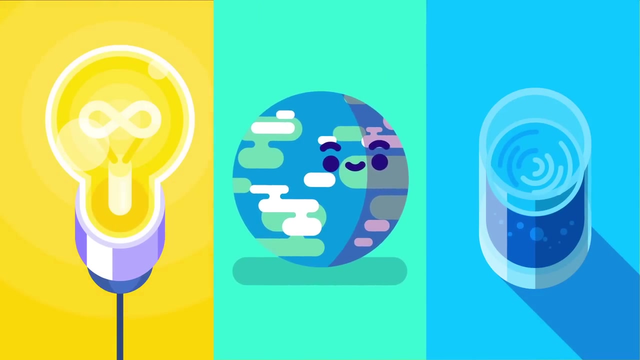 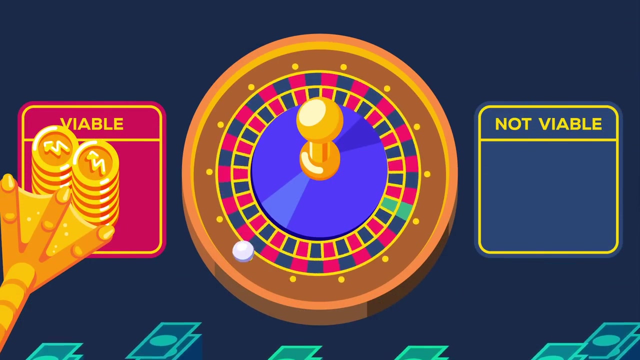 so a leak would be quickly diluted. So we've just told you that there's nearly unlimited energy to be had at no expense to the environment in something as simple as water. So what's the catch Cost? We simply don't know if fusion power will ever be commercially viable. Even if they work, they might be too expensive to ever build. The main drawback is that it's unproven technology, It's a $10 billion gamble and that money might be better spent on other clean energy that's already proven itself. 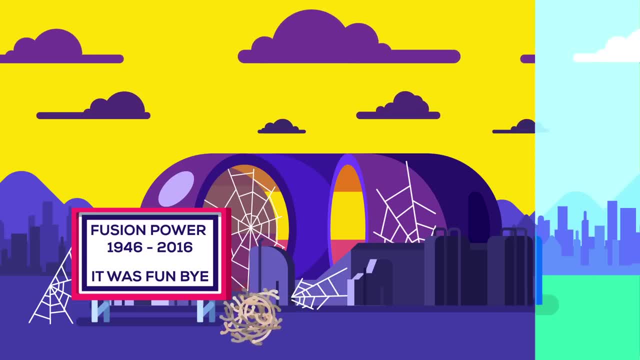 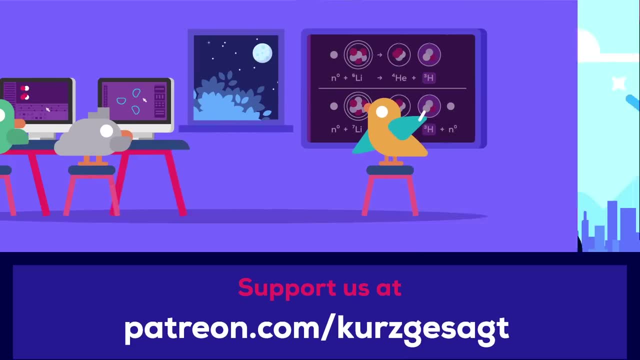 Maybe we should cut our losses. Or maybe, when the payoff is unlimited clean energy for everyone, it might be worth the risk. If you want to learn more about global energy, here's a playlist about nuclear energy, fracking and solar power. Let us know in the comments if there are other technologies you want us to explain.